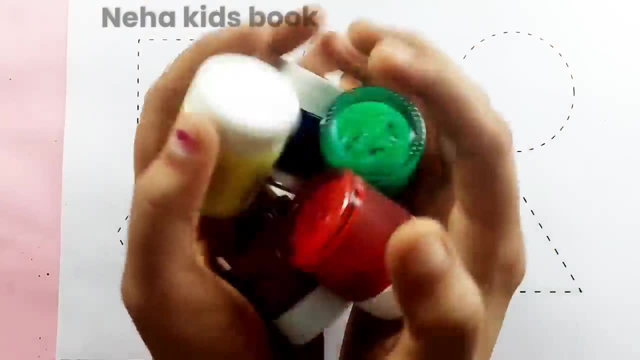 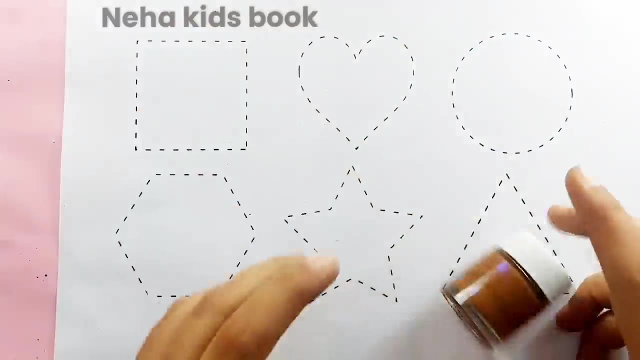 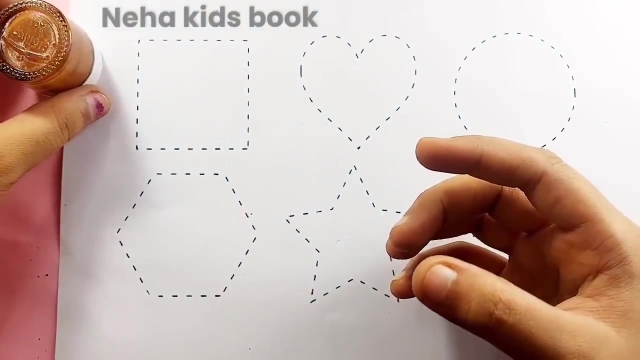 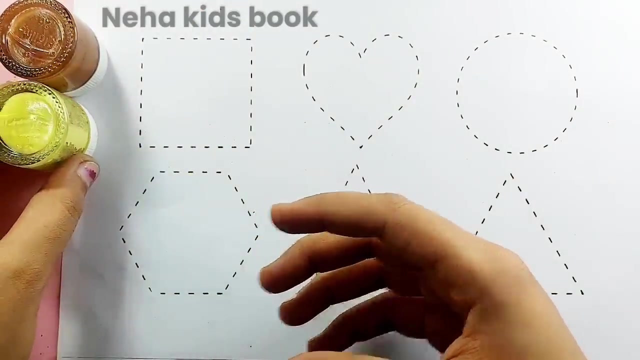 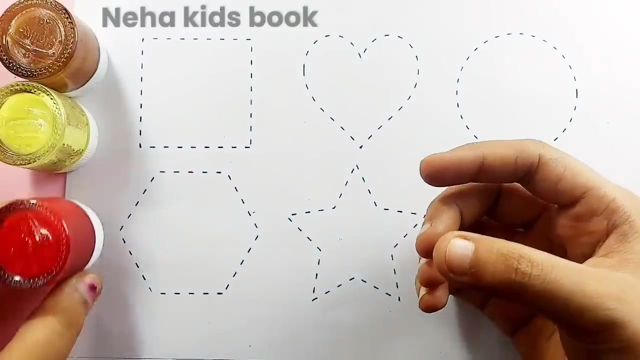 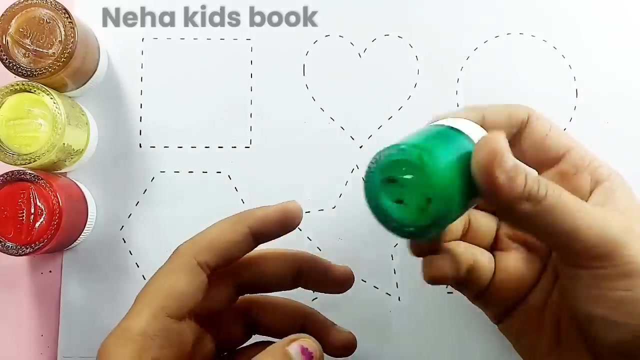 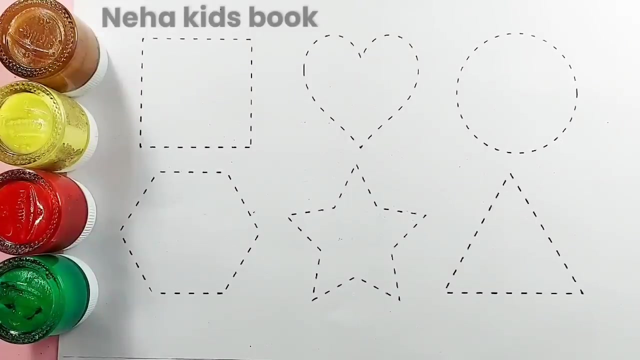 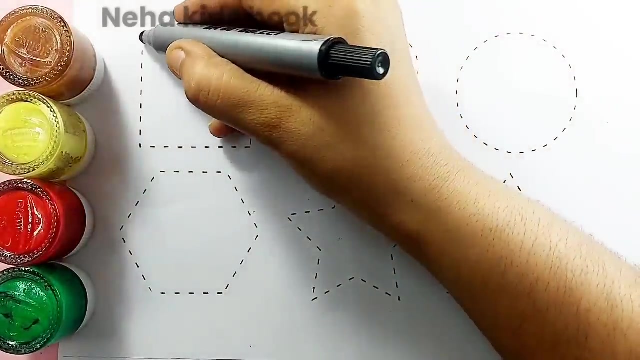 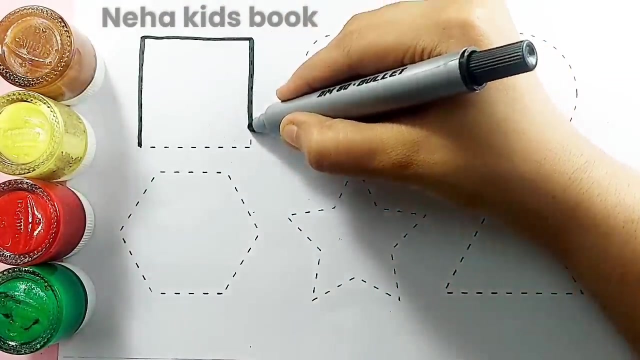 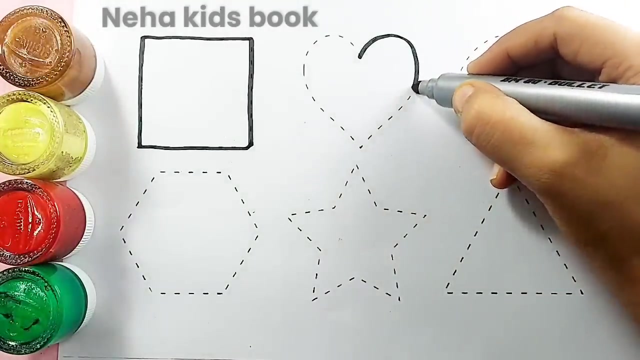 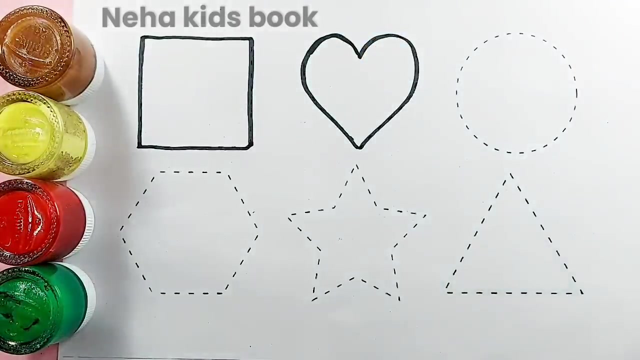 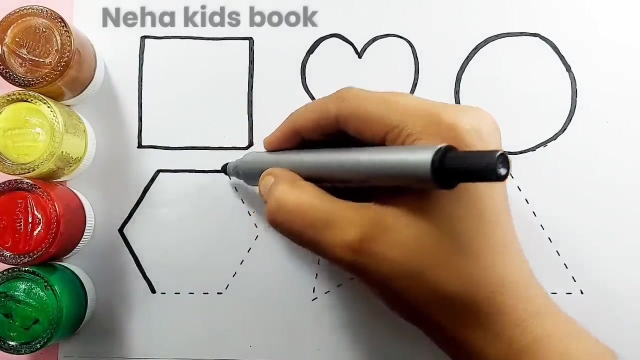 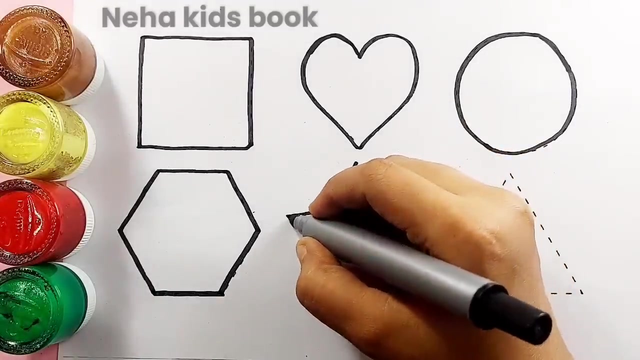 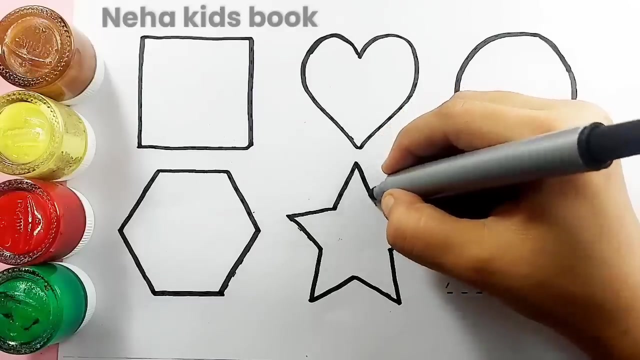 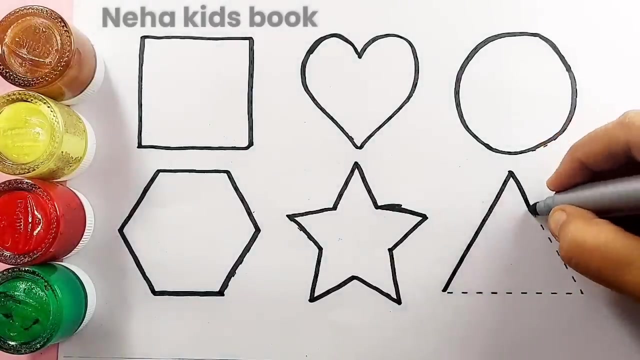 Brown color Brown color, Yellow color, Yellow color, Red color, Red color, Green color, Green color, Green color Circle Square Square Heart Heart Circle. Hexagon Star Star Triangle. Square Heart Circle- Hexagon Star Triangle. 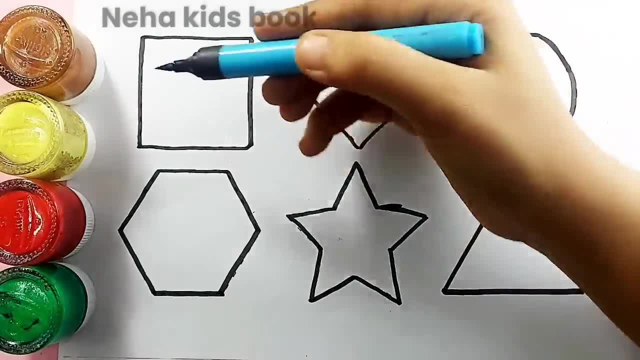 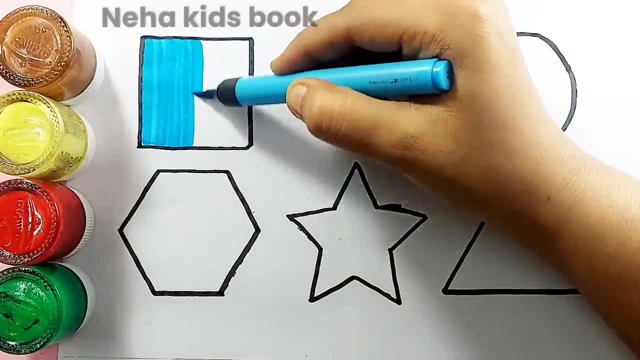 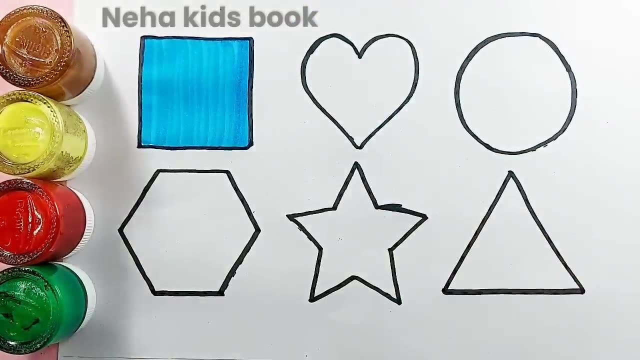 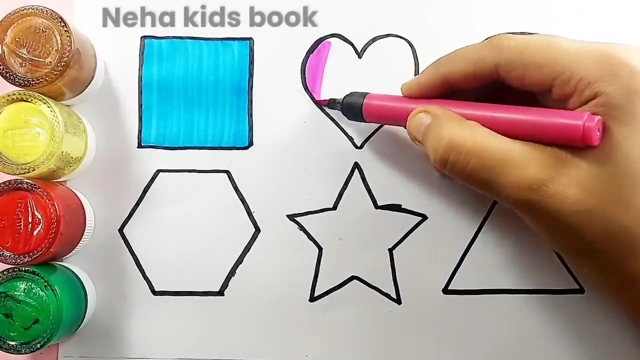 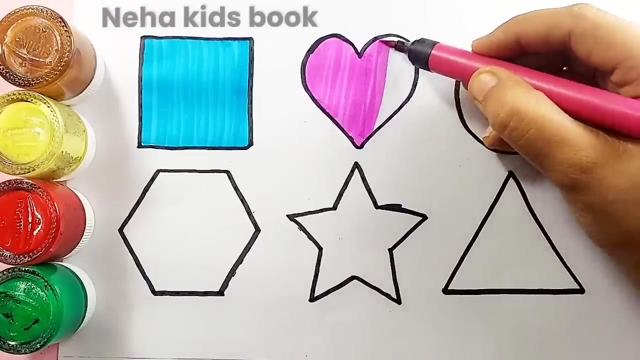 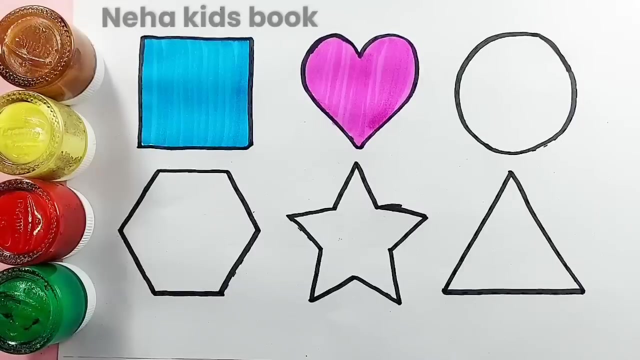 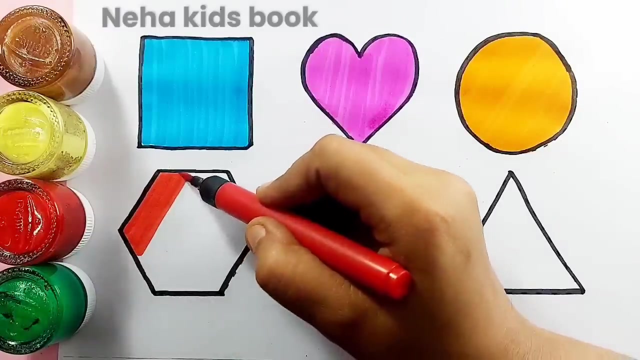 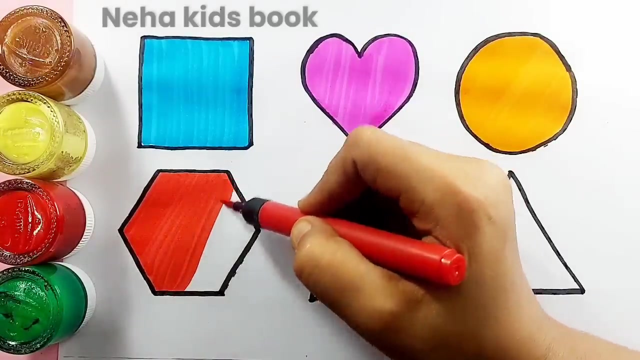 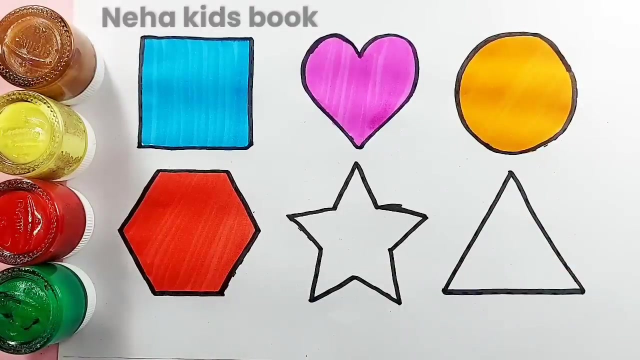 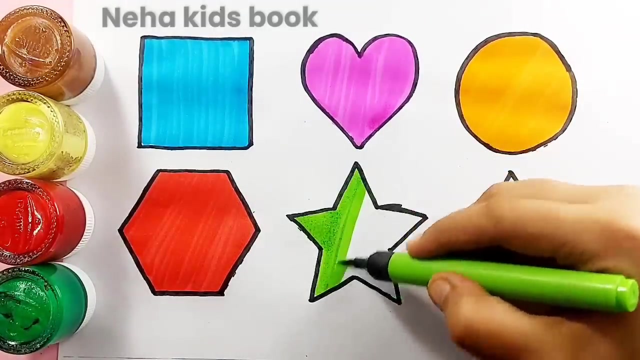 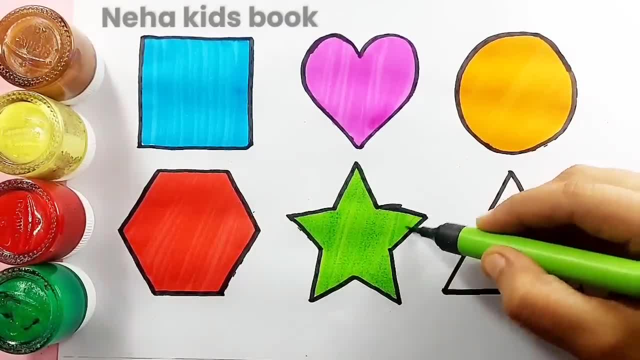 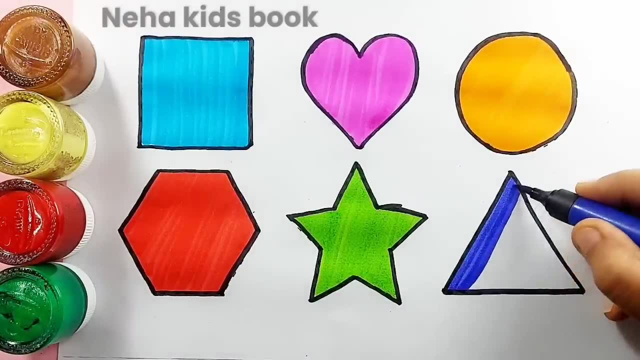 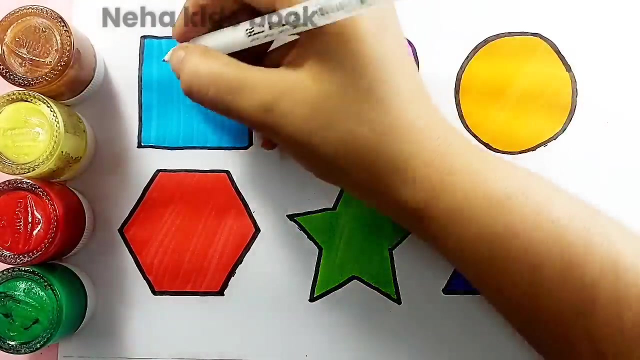 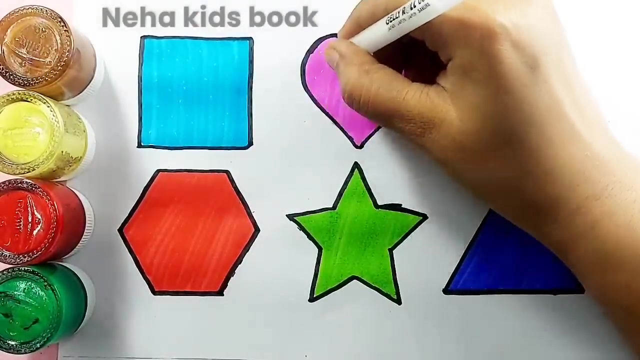 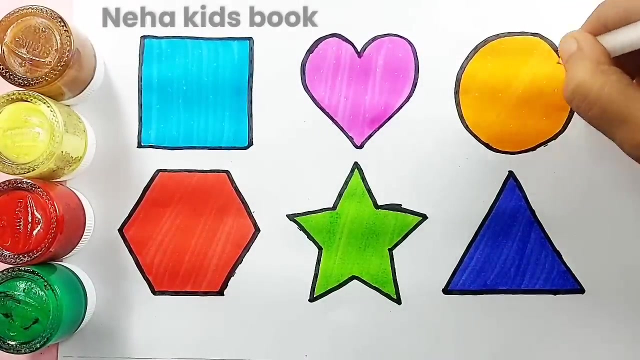 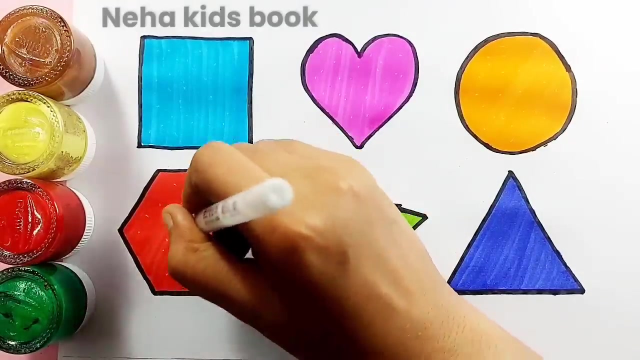 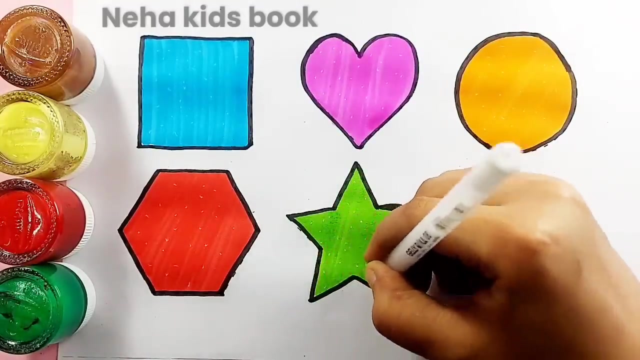 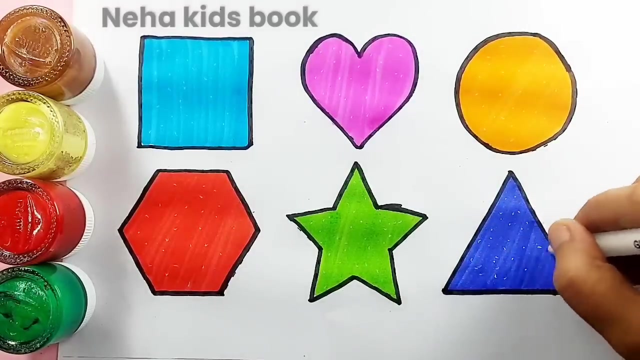 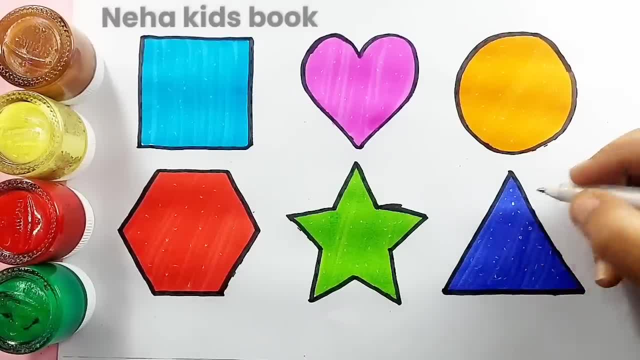 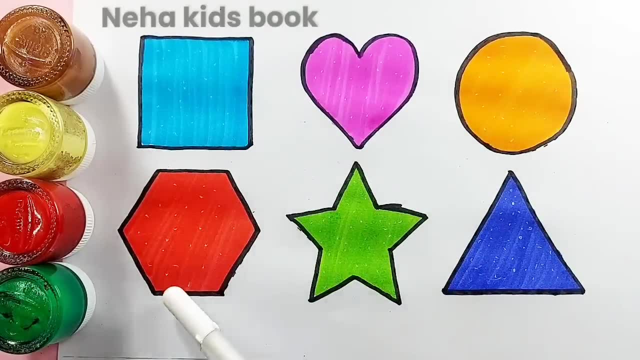 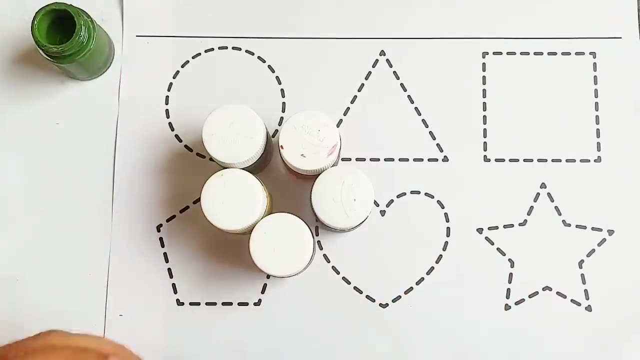 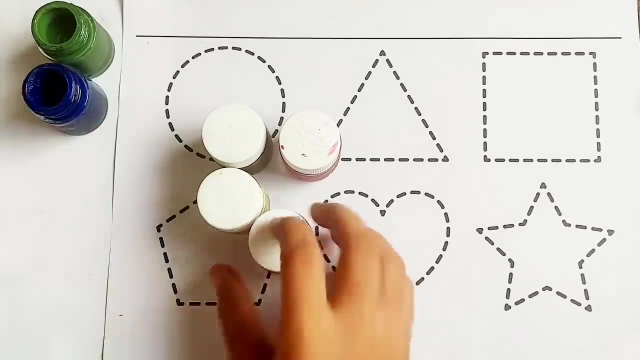 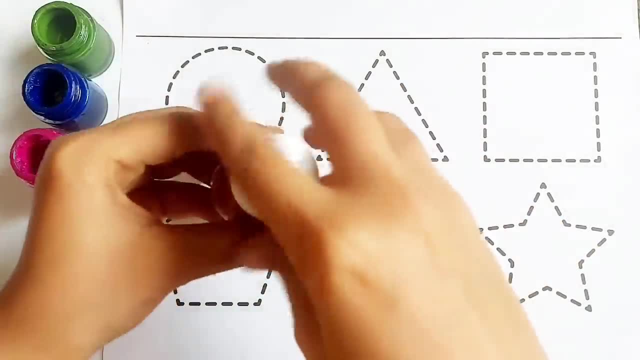 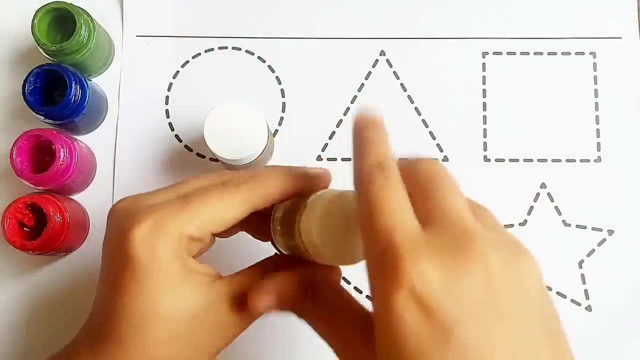 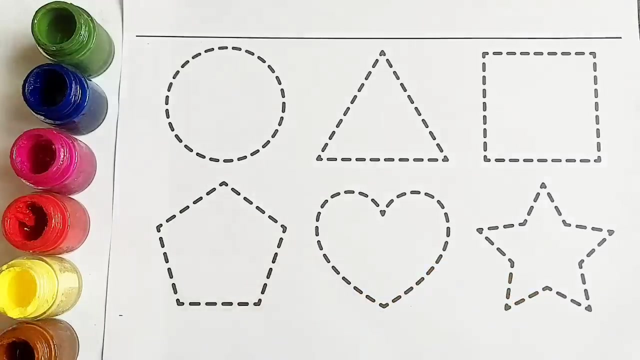 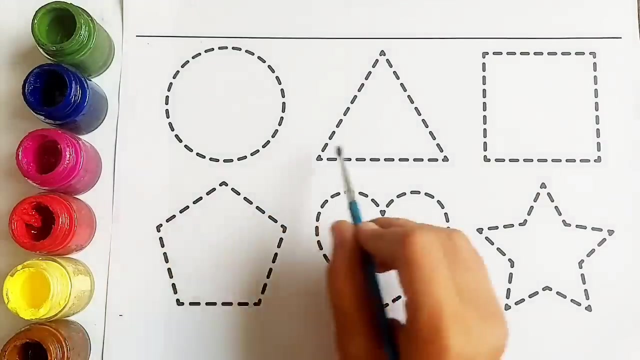 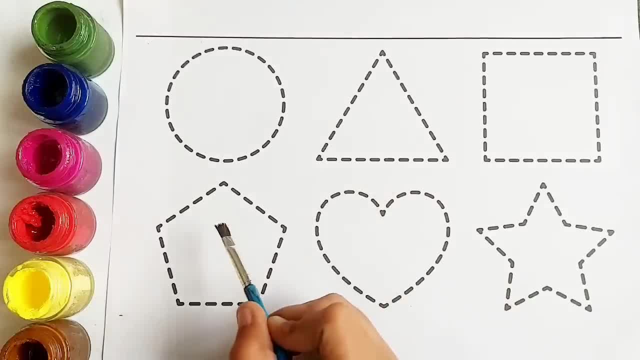 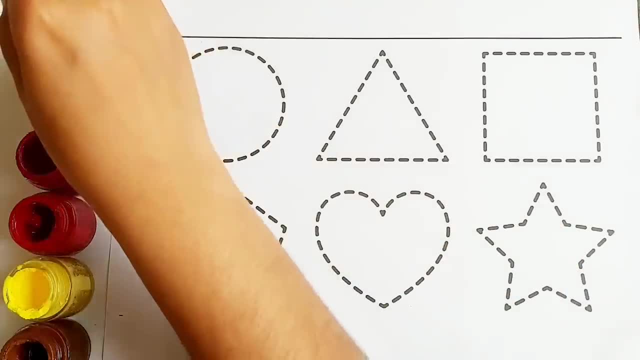 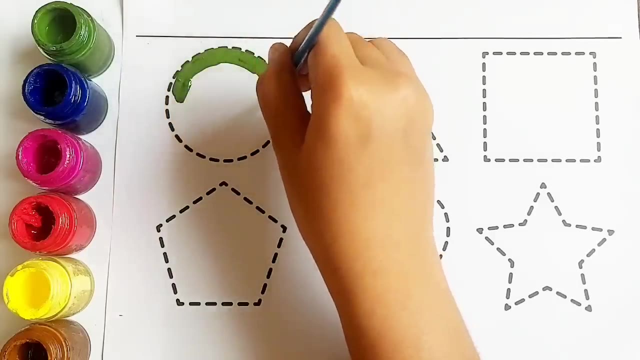 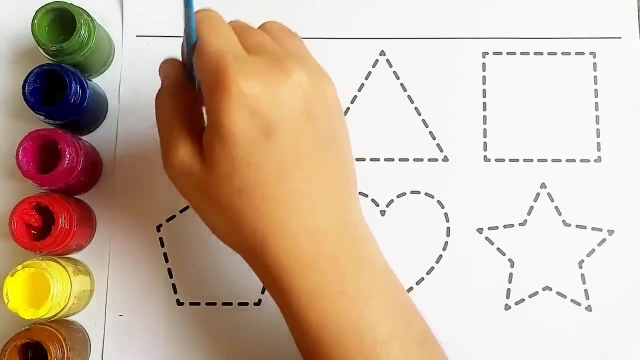 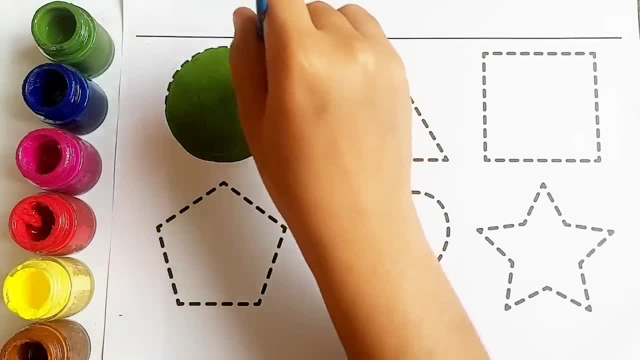 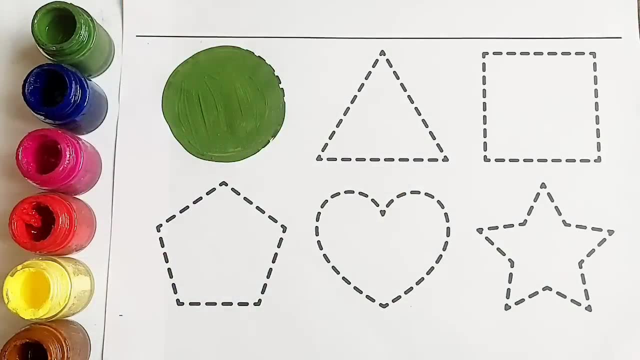 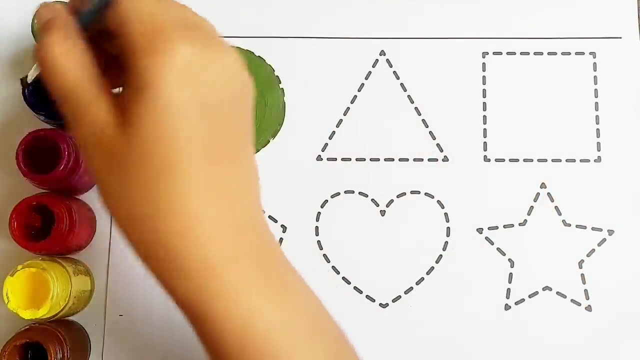 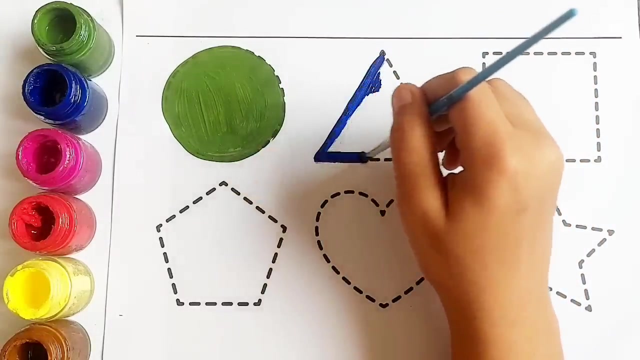 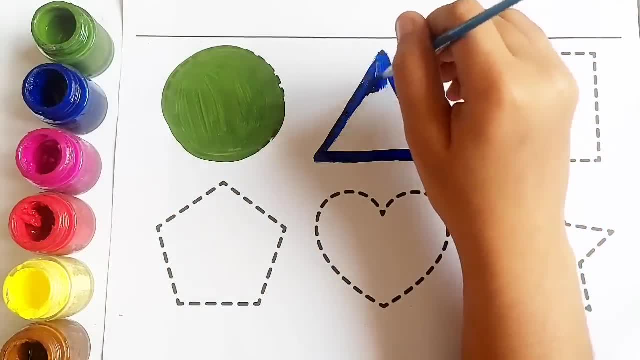 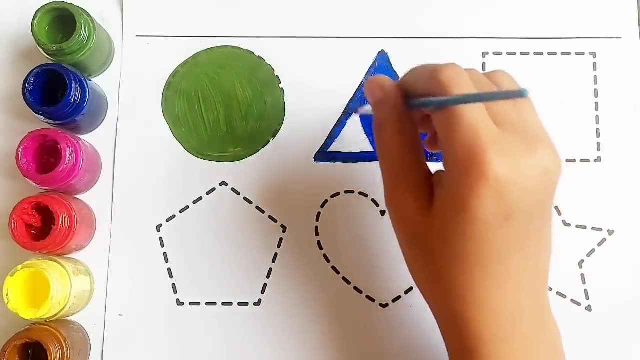 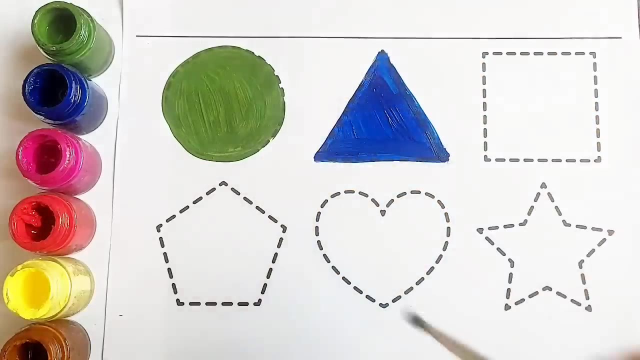 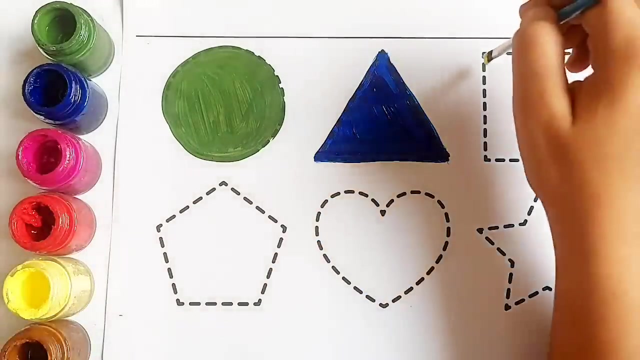 Triangle. Blue color Triangle- Blue color Triangle. Triangle Chali bicho. Next, kaunsa shape hai? Ye hai square Square. mein kaunsa color karenge? Yellow color. Yellow color. Yellow color Square. 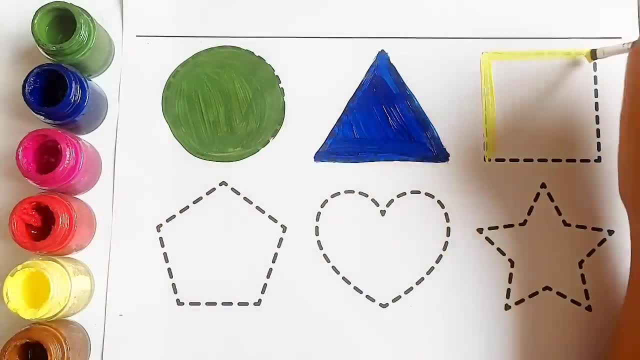 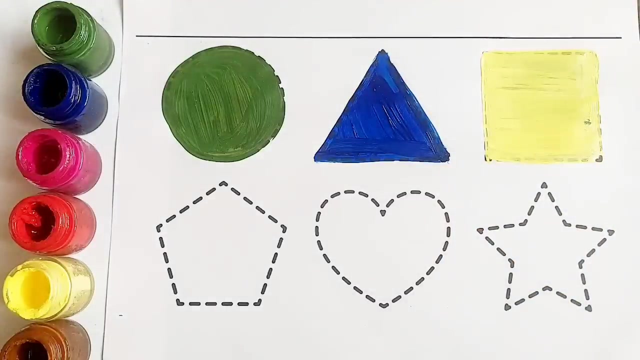 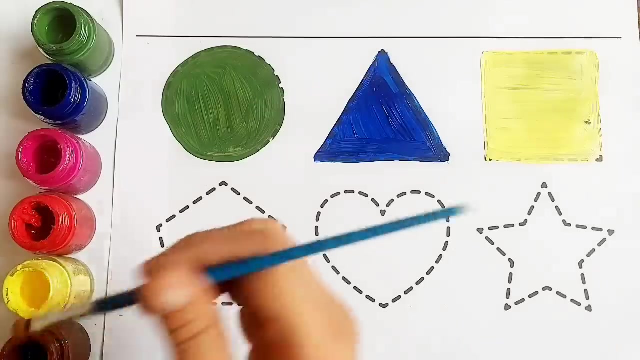 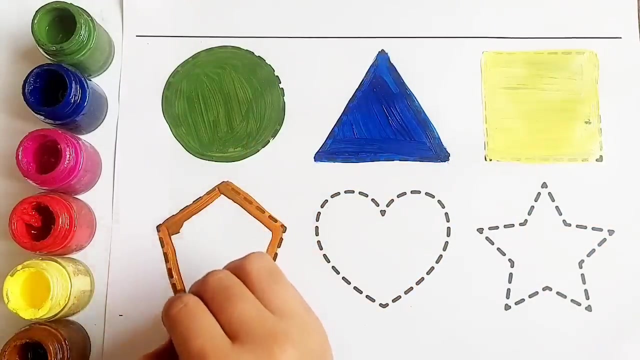 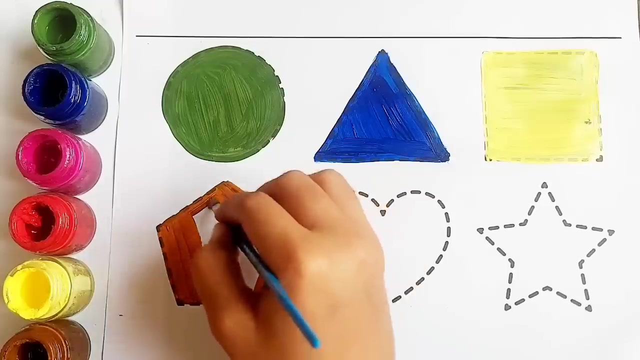 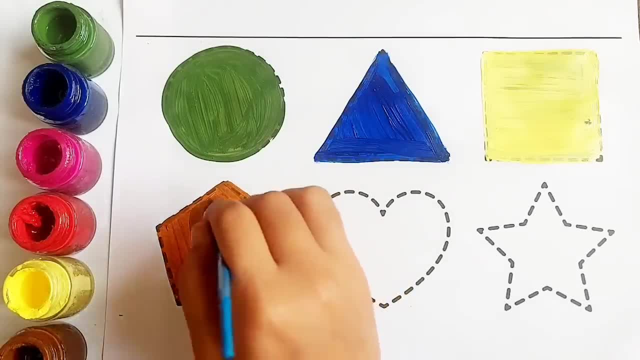 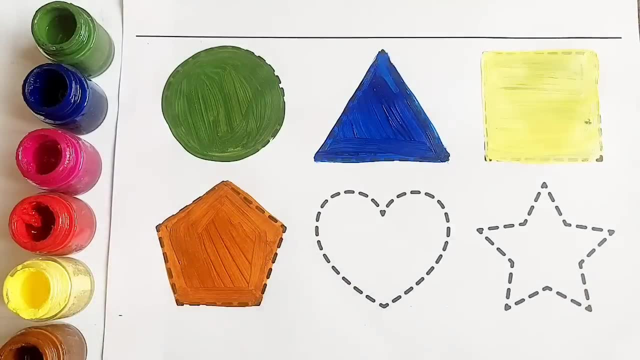 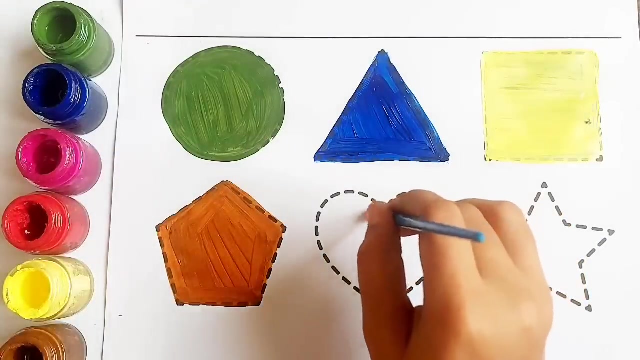 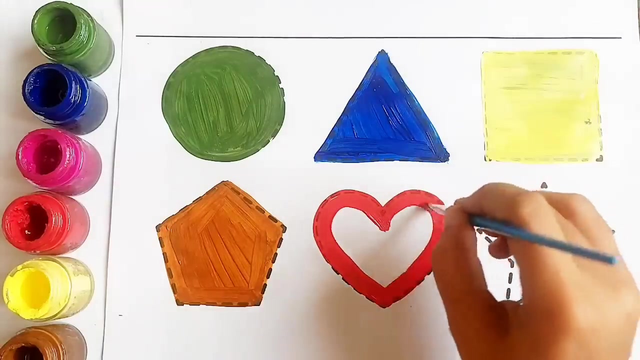 Yellow color. Bachcho, yeh kaunsa shape hai. Yeh hai pentagon. Next, kaunsa shape hai. bachcho, Yeh hai heart, Heart hai kaunsa color karenge? Red color, Heart, Red color, Heart, Heart, Red color. 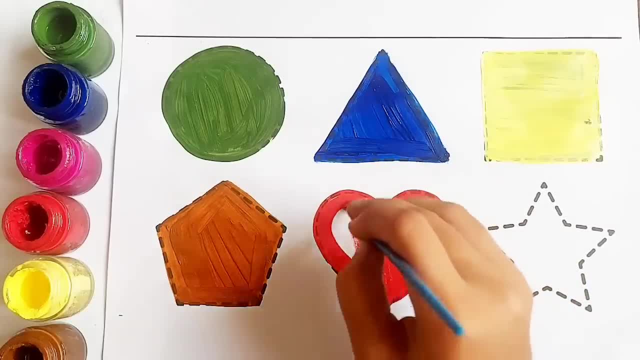 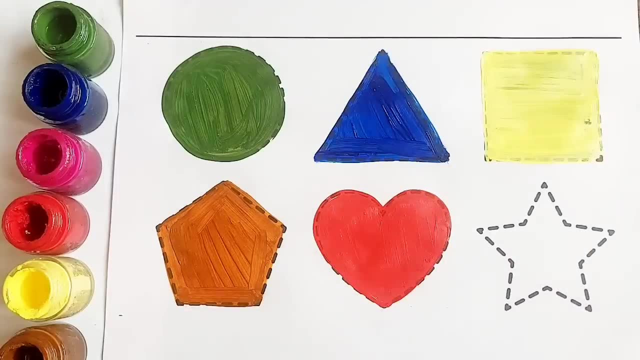 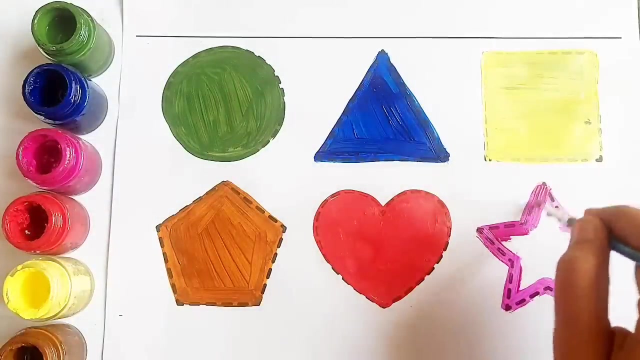 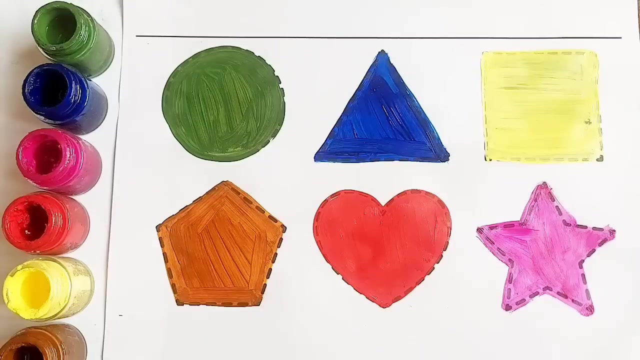 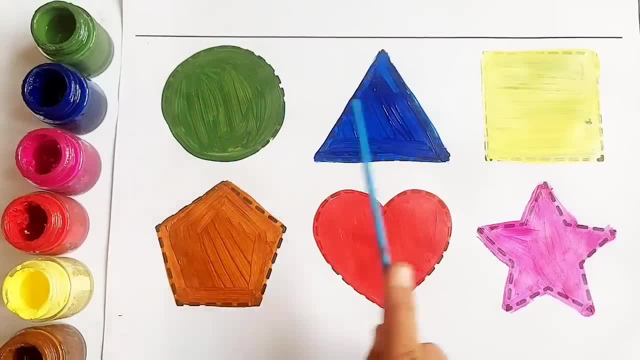 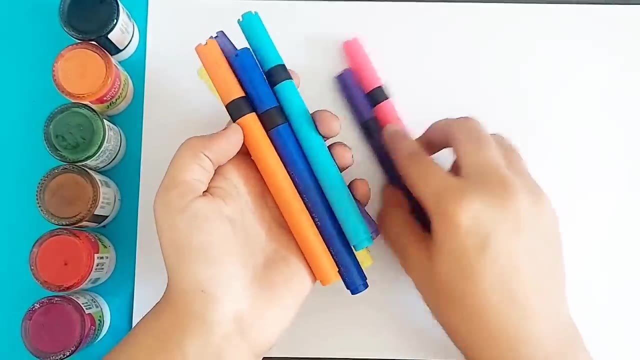 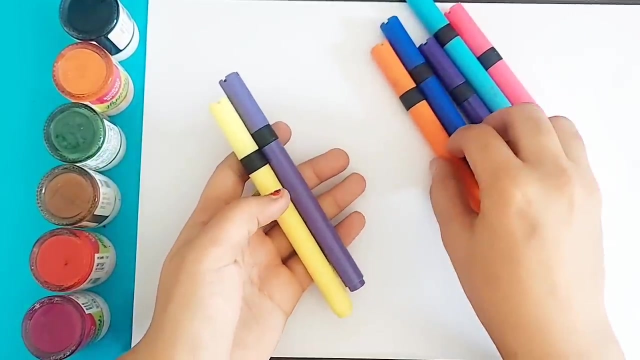 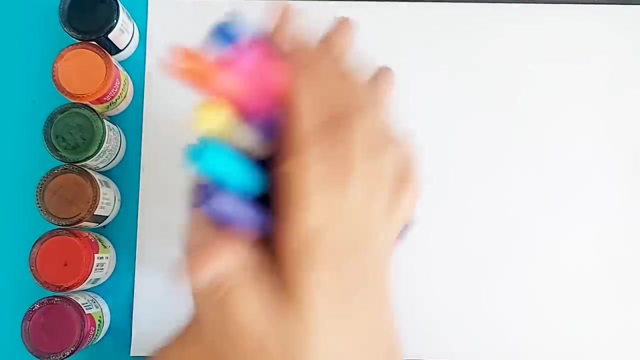 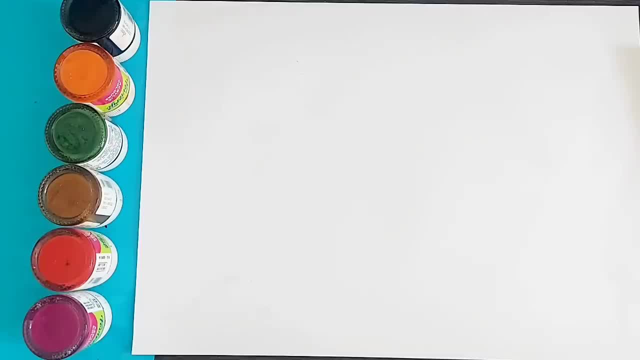 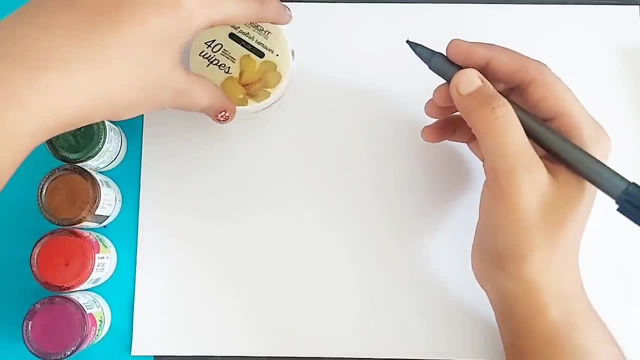 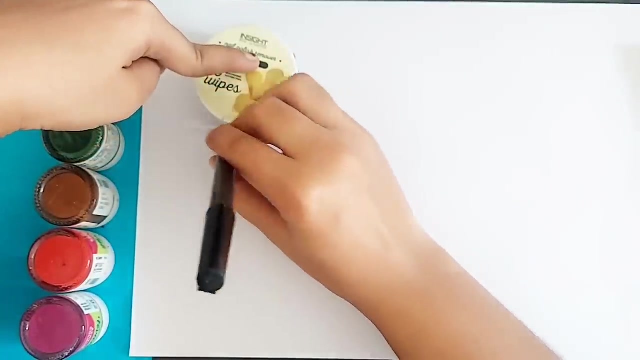 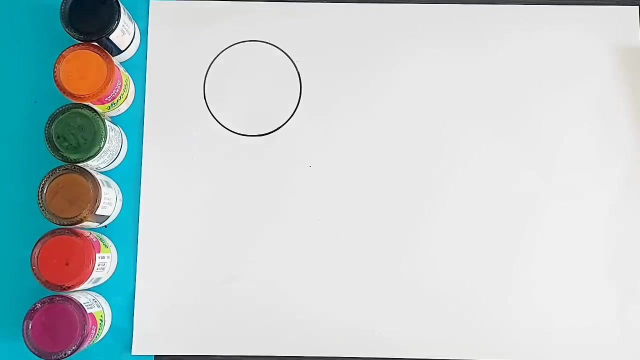 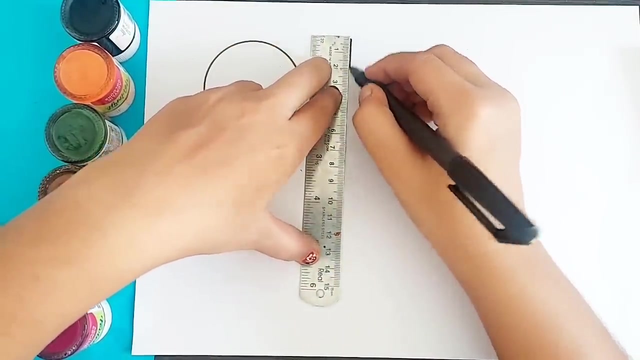 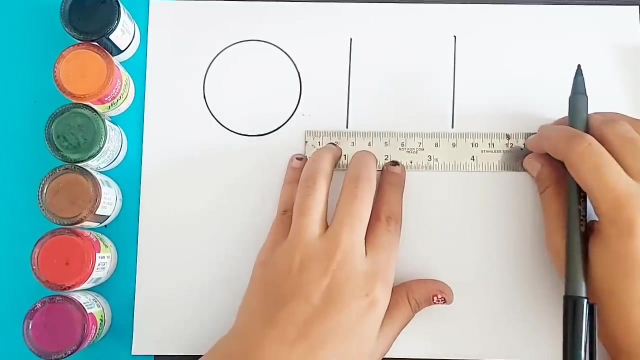 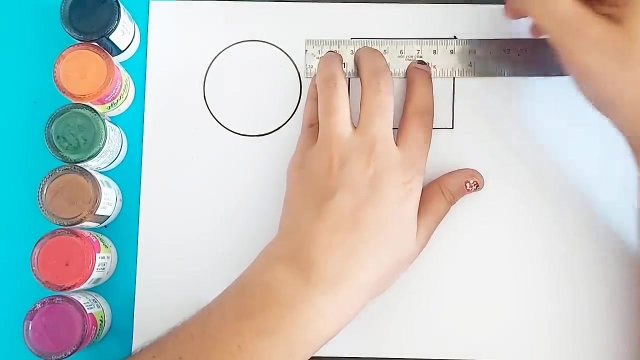 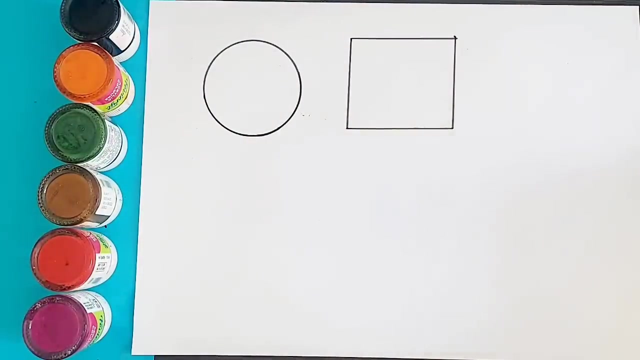 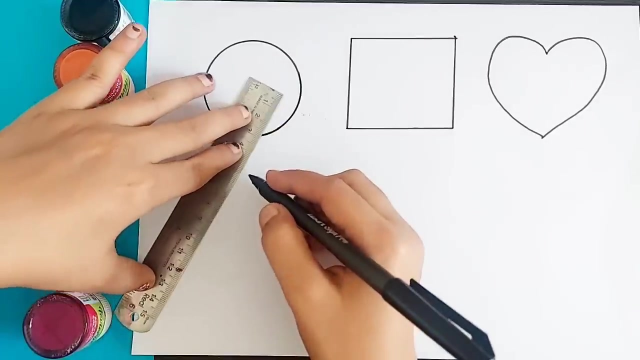 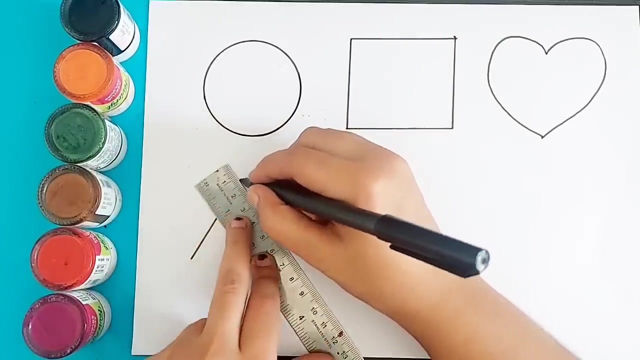 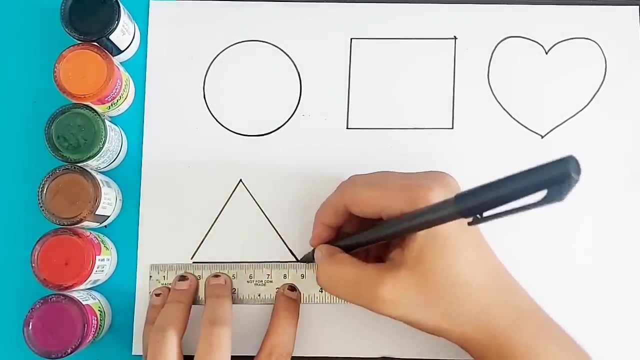 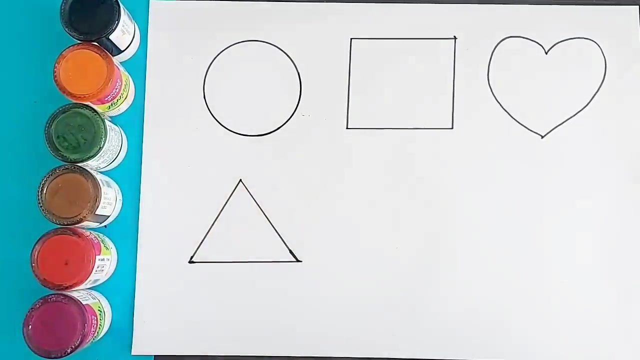 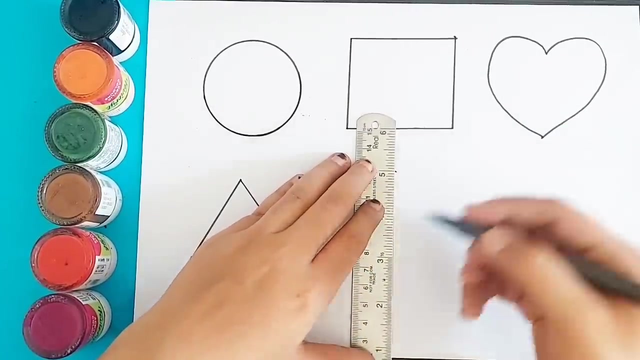 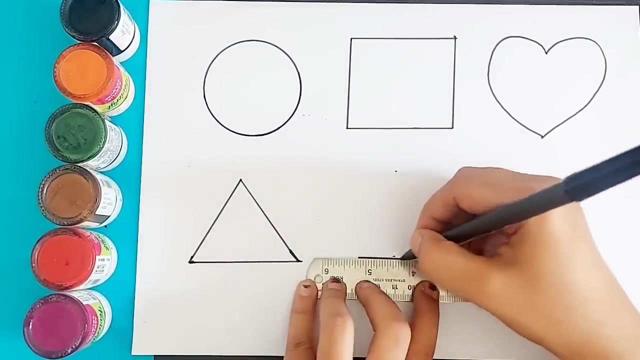 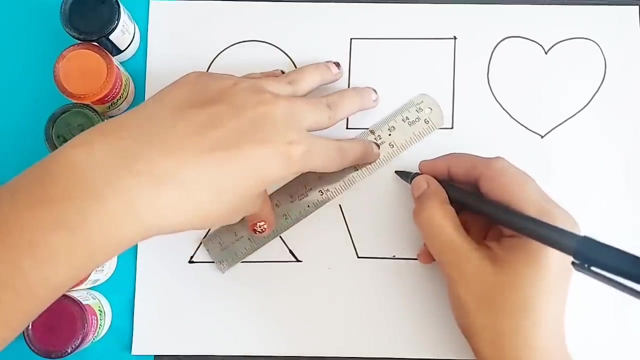 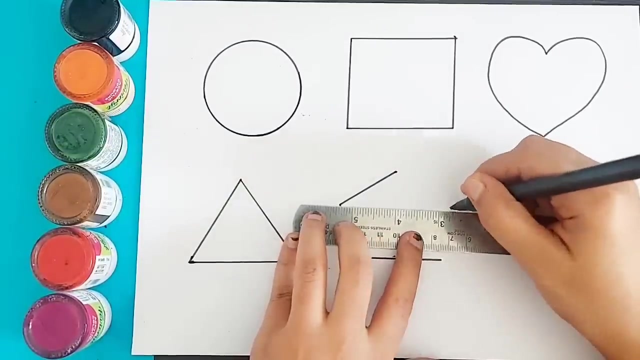 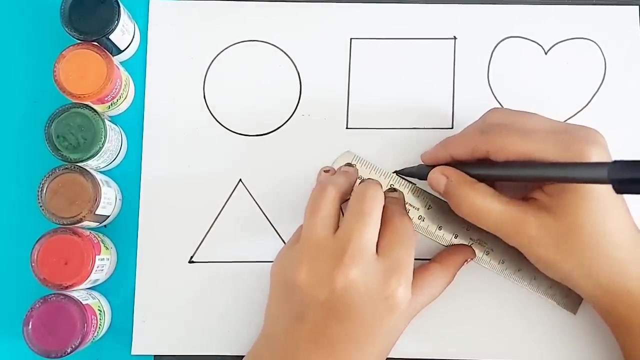 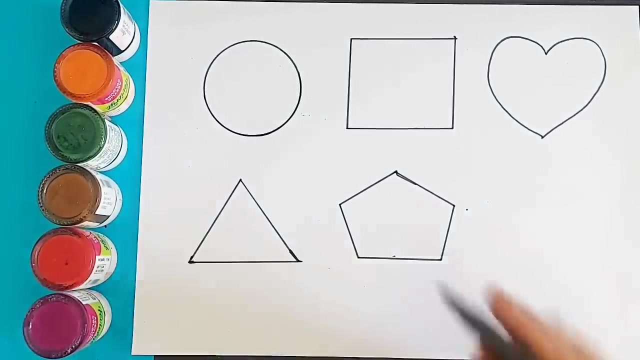 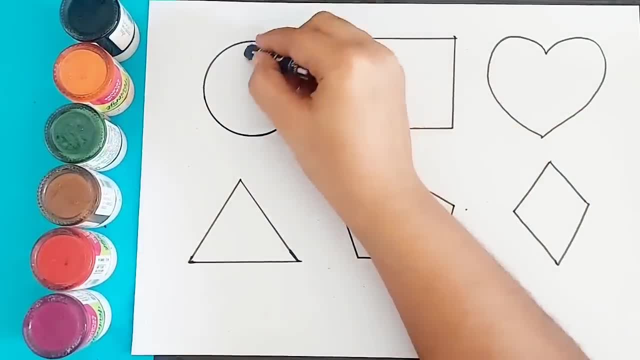 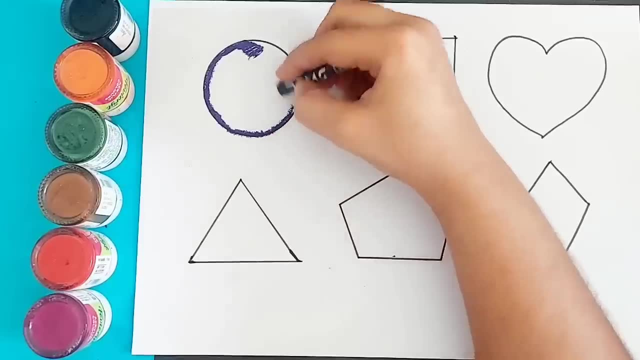 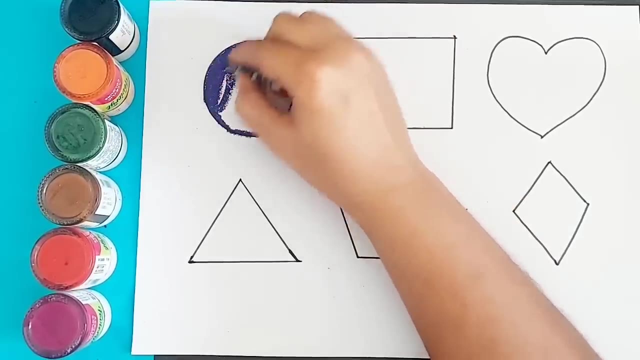 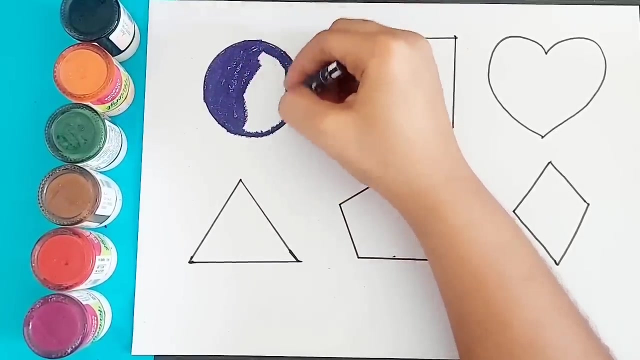 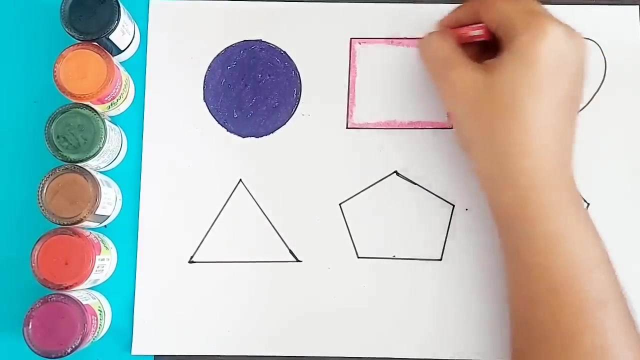 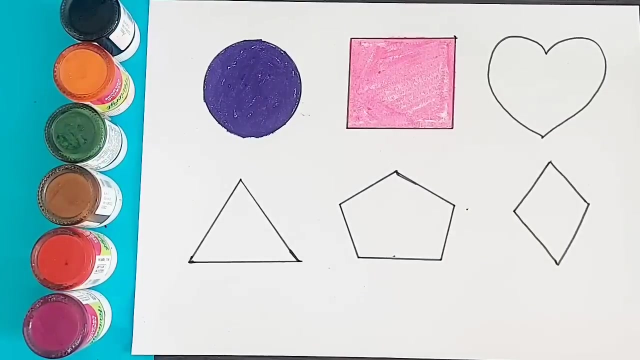 Violet color Circle. Violet color Circle. Violet color Circle. Pink color Square. Pink color Square. Pink color Square. Orange color Heart: Orange color Heart: Orange color Heart. Yellow color Triangle: Yellow color Triangle. Yellow color Triangle. Green color Pentagon. Green color Pentagon. Green color Pentagon. Red color Diamond. Red color Diamond. 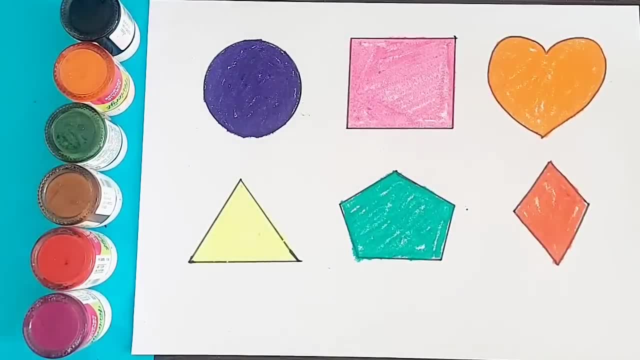 A, B, C, D, E, F, G, H, I, J, K, O, F, G, Q, R, S, T, U, V, W, M, X, Y, Z. Now I know my ABCs.